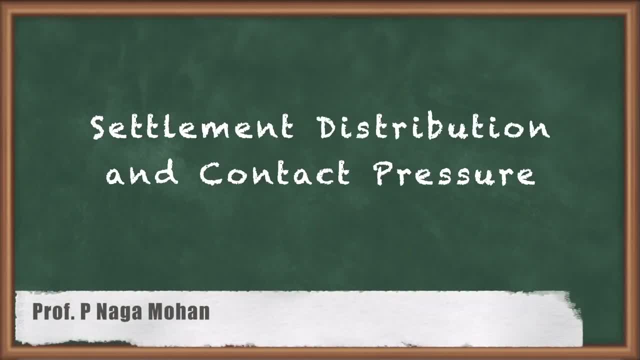 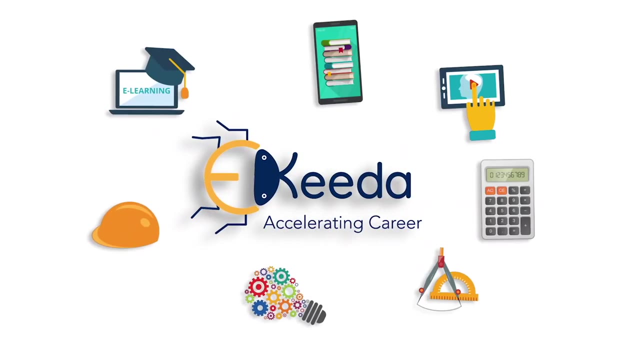 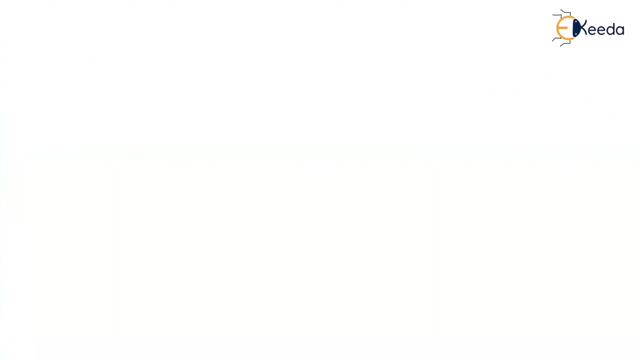 Hello friends, in the present video we will see how the contact pressure and settlement will occur along the width of a footing. So in the exam point of view it is not required how the magnitude will be, but it is required how the shape of the settlement and how the contact pressure will vary over the width. 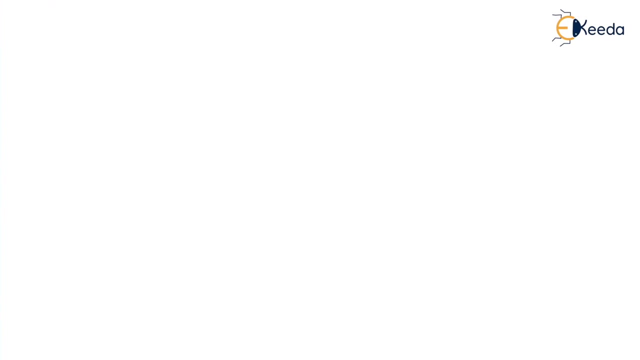 of a footing, if it is a flexible footing and also we have to see if it is a rigid footing. So for that let me write down here from the first I am writing: it is a flexible footing and second column, Rigid footing. 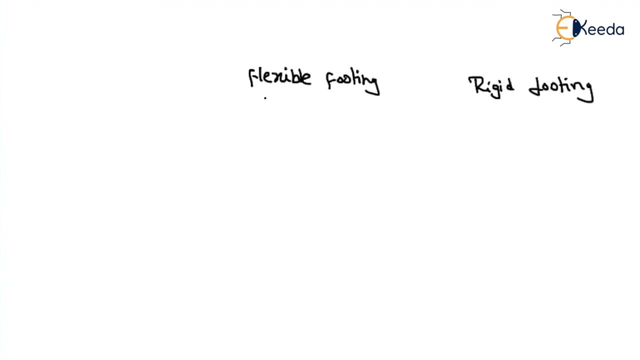 So let us first talk about the settlement and then we will see how the contact pressure will vary. Next let us say if it is a clayey soil and next it is considered a granular soil. So if it is a flexible footing granular soil, it is considered like this. you will 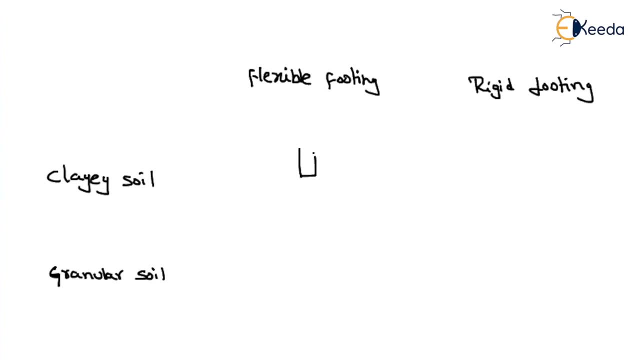 find the rested link of the soil, and if it is a flat footing it will suck and becomes flat. we will see how it is translated here. Next we will see the inclines, So such inclines are known as the iemand rega possiamo girdera are fiveettiukti soil. 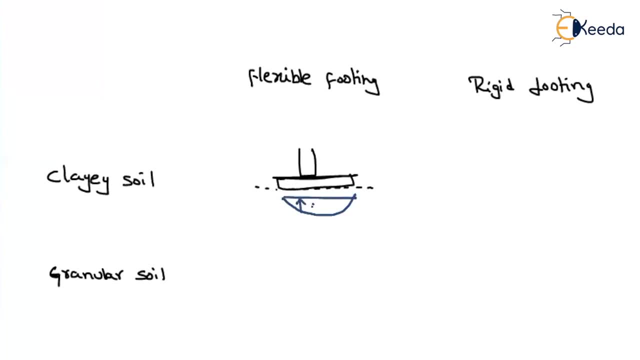 an inclinations will apply under the clayey soil If it is a filling granular soil. So minimum at the ends and maximum at the middle. Similarly, let us see in the rigid footing. If it is a rigid footing then we will have minimum at the center and maximum at the edges. 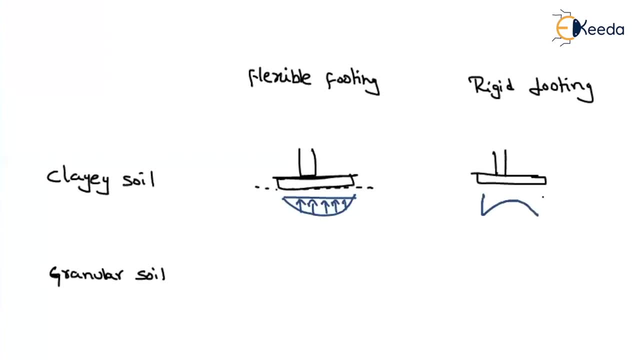 like this. See the variation. If it is a flexible footing for a clayey soil, settlement will be minimum at the edges, maximum will be at the center. If it is a rigid footing, maximum at the edges, minimum at the center. 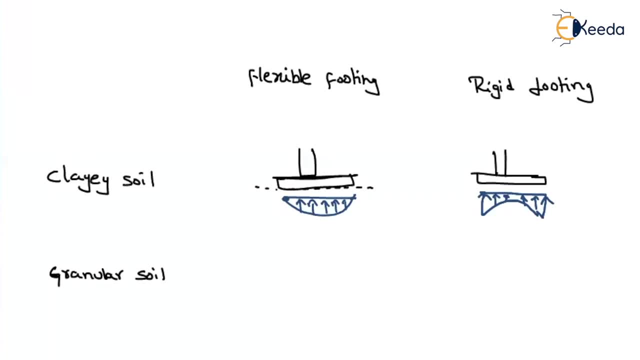 This is what is required for the gate exam. Similarly, let us see about the granular soil. If it is a granular soil on a flexible footing, then the settlement variation will be like this, So what it will be: Maximum at the edges, minimum at the center. Similarly, if it is on a rigid footing minimum at the edges minimum at the center. Similarly, if it is on a rigid footing minimum at the edges minimum at the center, If it is on a rigid footing minimum at the edges minimum at the center. 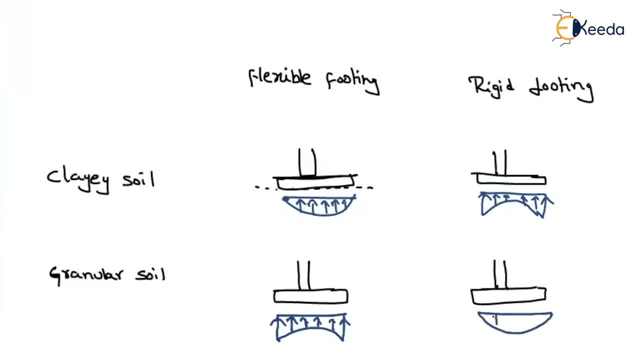 Then maximum at the edges, maximum at the center. So just opposite to each other, isn't it? Whatever, the settlement type of clayey soil will be opposite to the settlement pattern of granular soil. So if you can remember for one thing than you can remember for everything. just opposite. 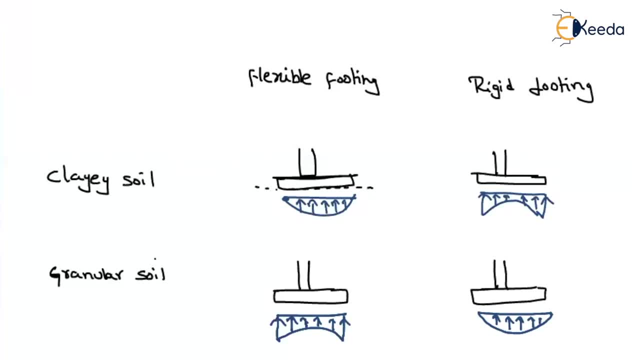 one. So if it is a clayey soil, let me remember one thing. and if it is a clayey soil, it is different from the other two. again. Well, the root is opposite from the nive smoothness. But then, on the south, ¡ find it. 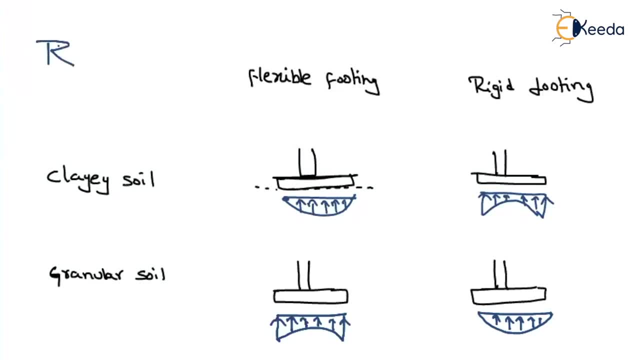 I will remember like this What is meant by R Rigid, isn't it? So there is a C portion, Is there or not? So rotate C in clockwise direction. Rotate C in clockwise direction. Now it will look like this shape: 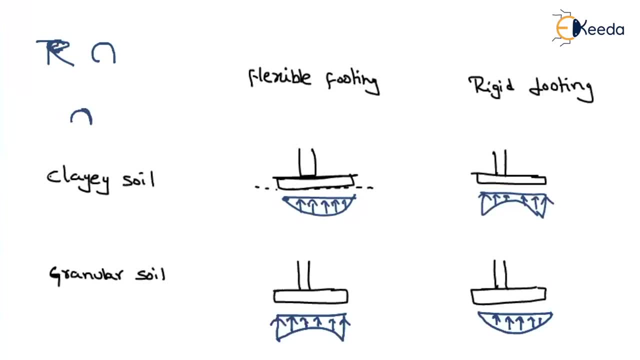 That means for rigid. we are having some C shape, And if we rotate C in clockwise the shape will become like this. Then it will be So. don't think that you will remember the pictures like this In exam. definitely we will get confused. 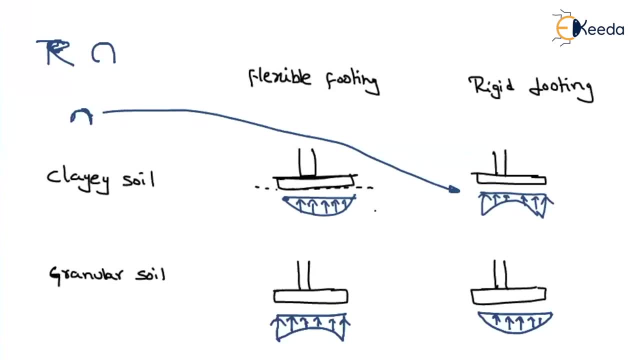 So we have to make some thumb rule. It's up to your wish. This is how I have remembered. If it is anything easy pattern, then you can remember that also. But remember whatever the thumb rule you will follow, but make sure that you will end up with the correct answer.